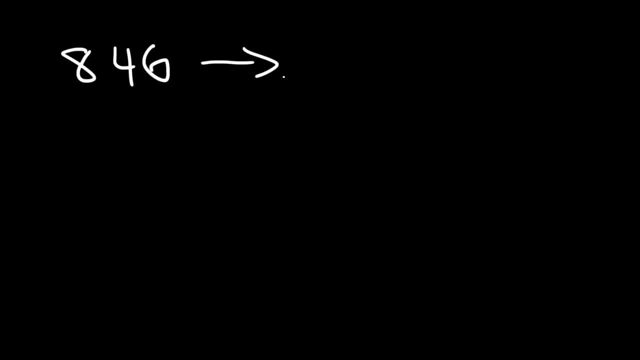 significant figures are there. Every non-zero number is a significant figure. So there's three significant figures in this number. Another example- 3546, has four significant figures. Now let's say, if we have a zero in between two non-zero numbers, Is that zero significant? All zeros between two non-zero numbers will. 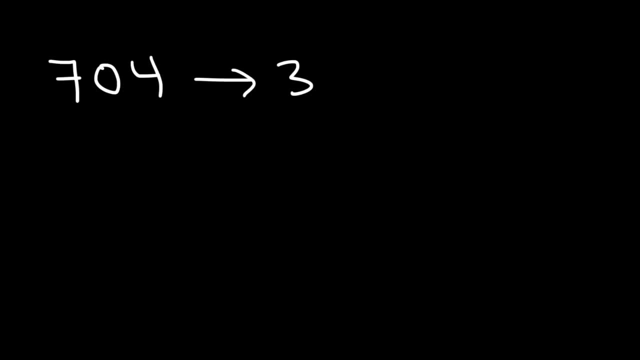 be significant. So 704 has three significant figures, 5006 has four significant figures. Now what about zeros to the right of a non-zero number like 500? How many significant figures are there in this number? It all depends on if there's a decimal point or not. If we do not have a decimal point, 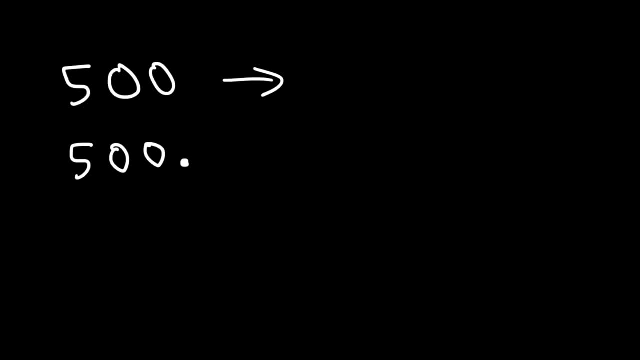 the zeros to the right, which are called trailing zeros, are not significant. Okay, So this would be only one significant figure. In this case, the trailing zeros are significant, So this would be three significant figures. Likewise, if we had 500.0, this would be four significant figures. Now what about the? 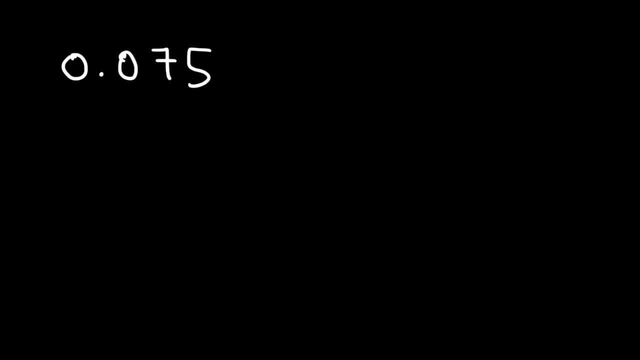 zeros to the left of a number like this .075?? Are these zeros the leading zeros? are they significant? Leading zeros are never significant. So there's only two significant figures: the seven and the five. So let's say, if we had .00836,, only these three. 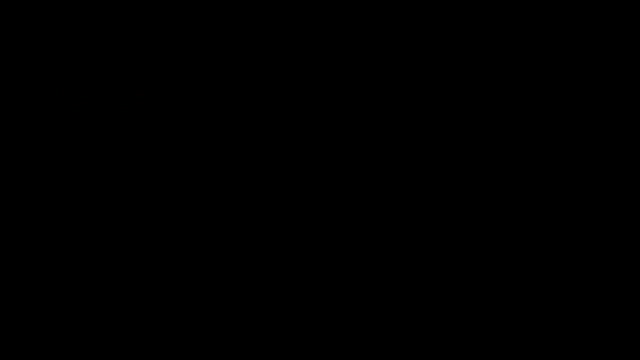 numbers will be significant. So to review, let's try this example: .0050830.. How many significant figures are in this number? So, looking at the leading zeros, remember the leading zeros are not significant. the zeros that are in between two non-zero numbers, those are significant and the trailing zeros are. 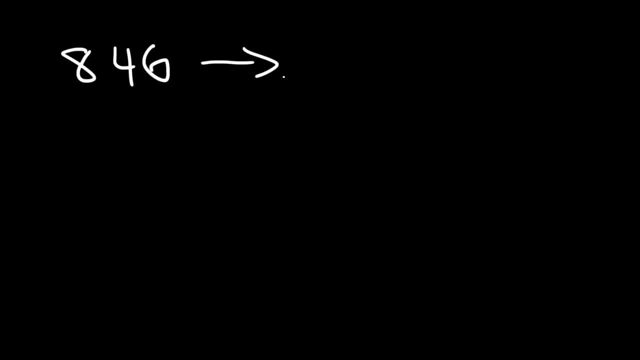 significant figures are there. Every non-zero number is a significant figure. So there's three significant figures in this number. Another example- 3546, has four significant figures. Now let's say, if we have a zero in between two non-zero numbers, Is that zero significant? All zeros between two non-zero numbers will. 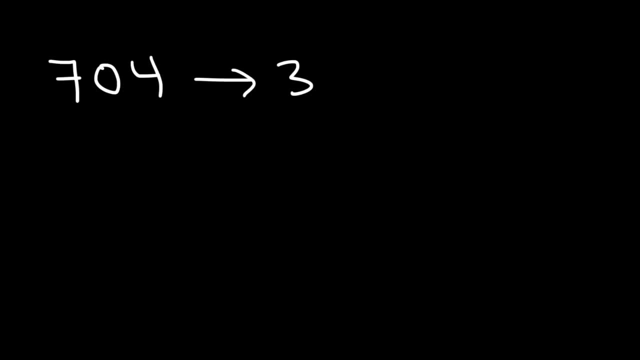 be significant. So 704 has three significant figures, 5006 has four significant figures. Now what about zeros to the right of a non-zero number like 500? How many significant figures are there in this number? It all depends on if there's a decimal point or not. If we do not have a decimal point, 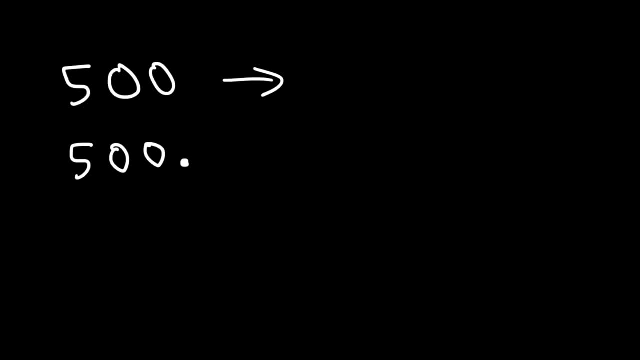 the zeros to the right, which are called trailing zeros, are not significant. Okay, So this would be only one significant figure. In this case, the trailing zeros are significant, So this would be three significant figures. Likewise, if we had 500.0, this would be four significant figures. Now what about the? 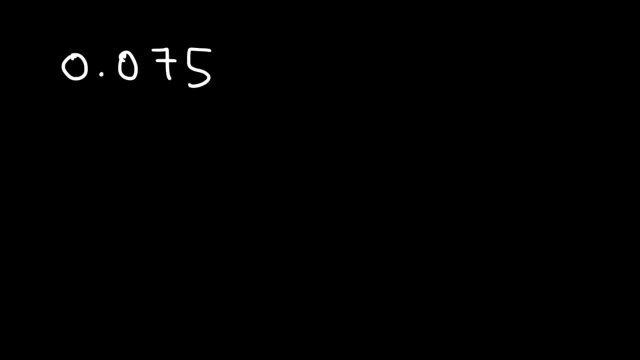 zeros to the left of a number like this, .075?. Are these zeros the leading zeros? are they significant? Leading zeros are never significant. So there's only two significant figures: the seven and the 5.. So let's say, if we had .00836,, only these three. 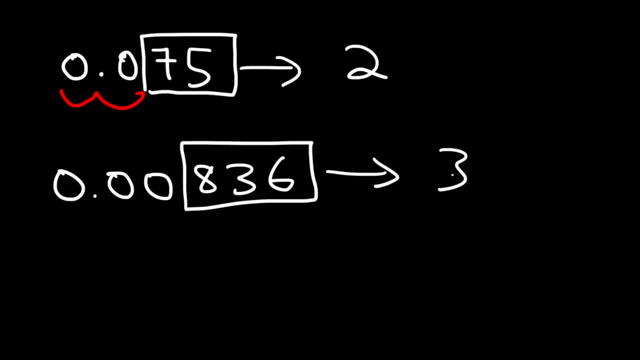 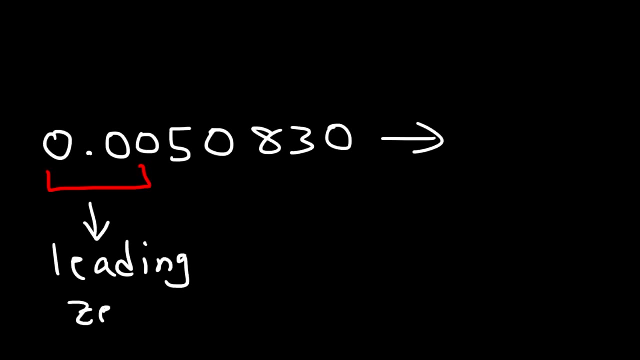 numbers will be significant. So to review, let's try this example: .0050830.. How many significant figures are in this number? So, looking at the leading zeros, remember the leading zeros are not significant. the zeros that are in between two non-zero numbers, those are significant and the trailing zeros are. 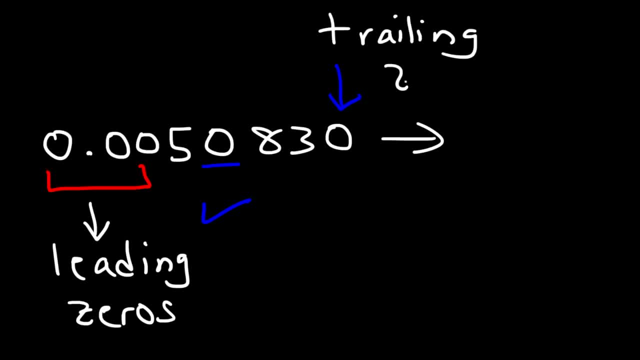 only significant if there is a decimal point, which we do have. so therefore, these five digits are significant. so we're going to have five significant figures. so what I'm going to do at this point is give you a quiz, and I want you to determine how many significant figures are in the following numbers. so 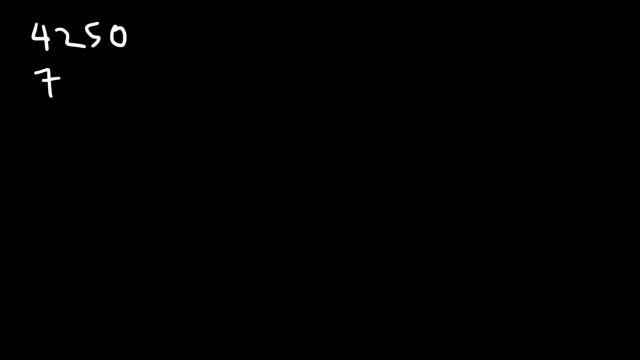 the first one is going to be 42, 50, and the second one is 7080, and then 30,000, 50 with a decimal point, and then .00703. next we have .08060 and then 5030.0 and finally 750.064080. go ahead and determine the number of significant. 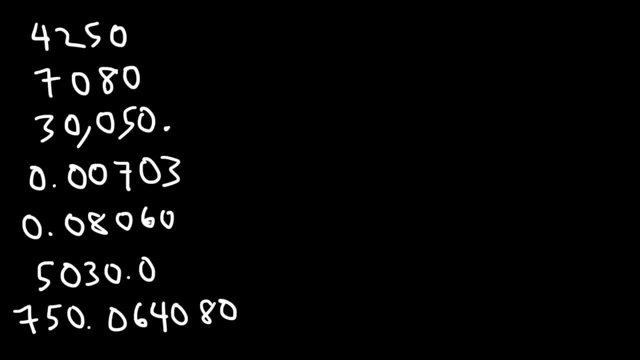 figures in each of those numbers. by the way, for those of you who want harder examples, or maybe just more examples, I have another video on YouTube that is about an hour and a half long, but it really goes deep into this topic. so, for those of you who want to master the concept of sig figs, you can. 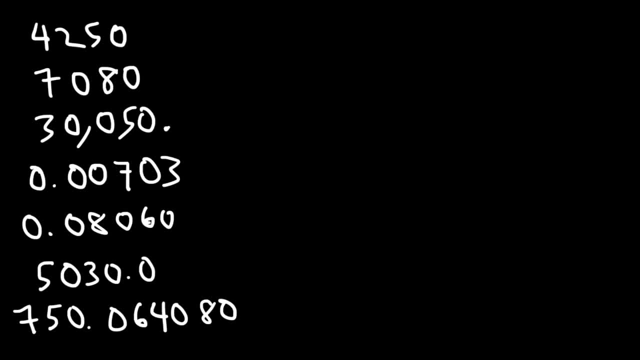 check out that video. I'm going to post the link in the description section of this video, so feel free to take a look at that when you get a chance. also, if you're going to subscribe to this channel, make sure to click the notification bell if you want to receive any updates. 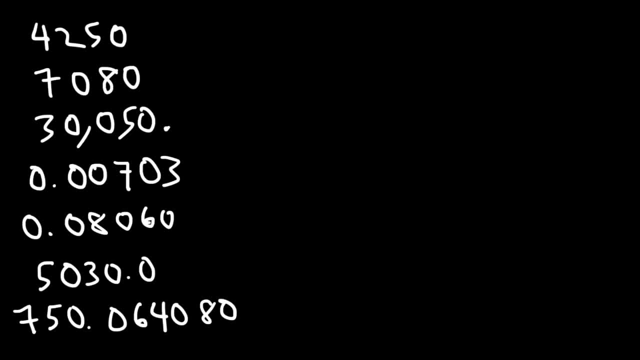 of any new videos that I'm going to post in the future, so let's go ahead and begin. so 4250, how many significant figures does it have? so the zero at the right do we count it? well, it's a trailing zero and there is no decimal point, so we're not going to. 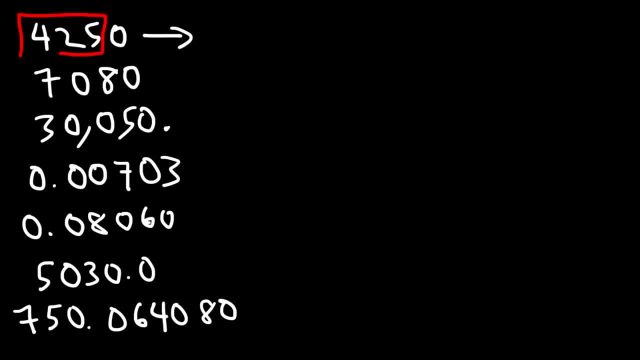 count it. so therefore, we can only count these three non-zero numbers. so we have three significant figures in the first example. now, what about the second example? how many significant figures are there? once again, we don't have a decimal point, so we cannot count that zero. but what? 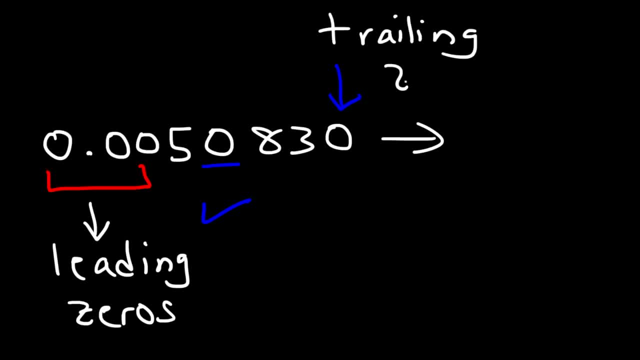 only significant if there is a decimal point, which we do have. so therefore, these five digits are significant. so we're going to have five significant figures. so what I'm going to do at this point is give you a quiz, and I want you to determine how many significant figures are in the following numbers. so 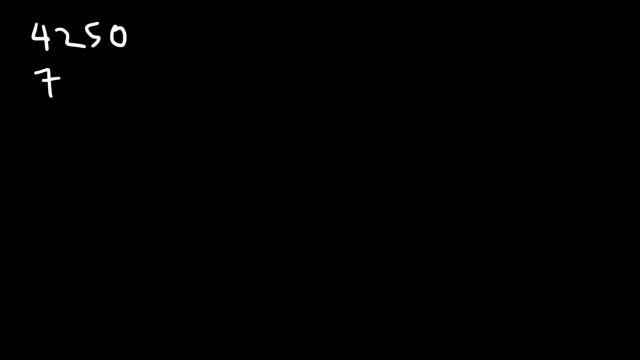 the first one is going to be 42, 50, and the second one is 7080, and then 30,000, 50 with a decimal point, and then .00703. next we have .08060 and then 5030.0 and finally 750.064080. go ahead and determine the number of significant. 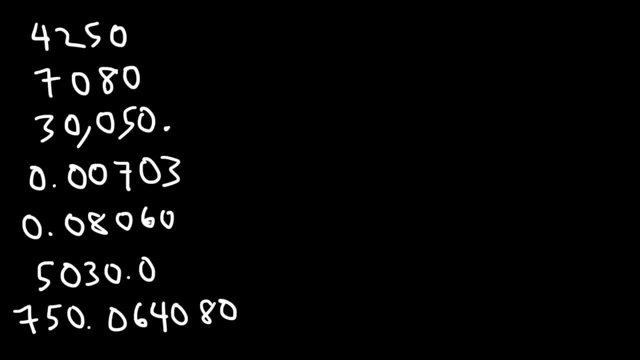 figures in each of those numbers. by the way, for those of you who want harder examples, or maybe just more examples, I have another video on YouTube that is about an hour and a half long, but it really goes deep into this topic. so, for those of you who want to master the concept of sig figs, you can. 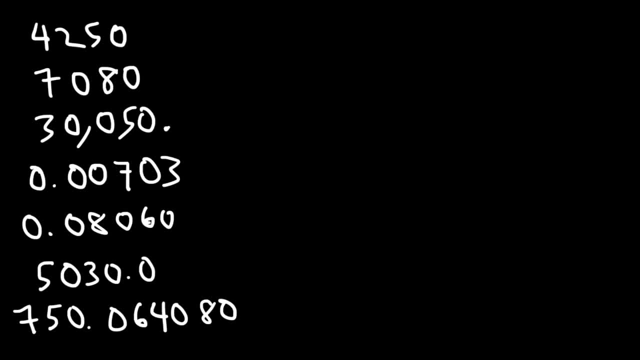 check out that video. I'm going to post the link in the description section of this video, so feel free to take a look at that when you get a chance. also, if you're going to subscribe to this channel, make sure to click the notification bell if you want to receive any updates. 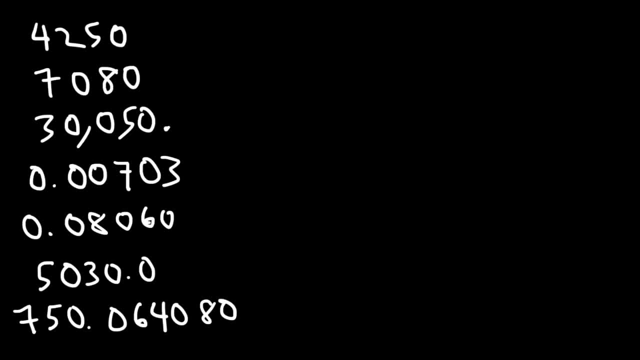 of any new videos that I'm going to post in the future, so let's go ahead and begin. so 4250, how many significant figures does it have? so the zero at the right do we count it? well, it's a trailing zero and there is no decimal point, so we're not going to. 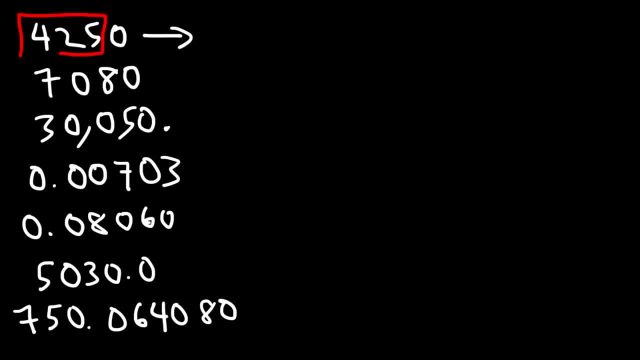 count it. so therefore, we can only count these three non-zero numbers. so we have three significant figures in the first example. now, what about the second example? how many significant figures are there? once again, we don't have a decimal point, so we cannot count that zero. but what? 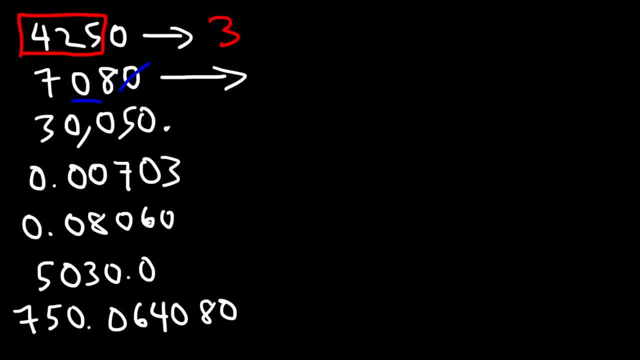 about the zeros in between non-zero numbers. so those zeros we can count. so therefore this answer- I mean this problem- also have a three significant figures. now for the next one. there is a decimal point, so the trailing zero is counted and all of the zeros in between the three and 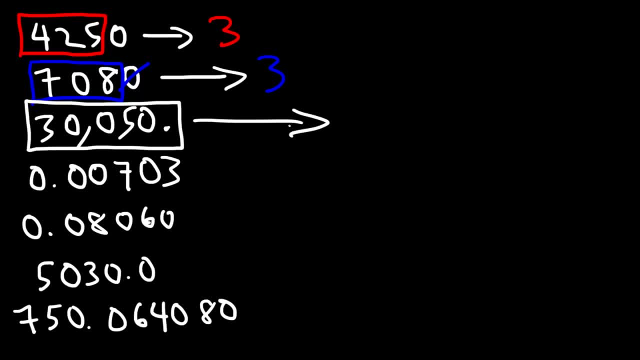 five are also counted. so this example is going to have five significant figures. for the next one, we do have a decimal point, but there are no trailing zeros. we do have some leading zeros, but those will not be counted, so only these three digits will be counted. so there's three significant figures in that number. 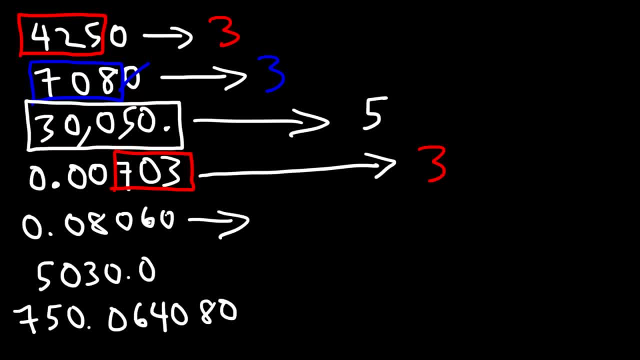 for the next one, we do have a trailing zero which will be counted. the leading zeros will not be counted, so there's only four significant figures now. in the next number, 5030, we have a decimal point, so all of the trailing zeros will be counted, and 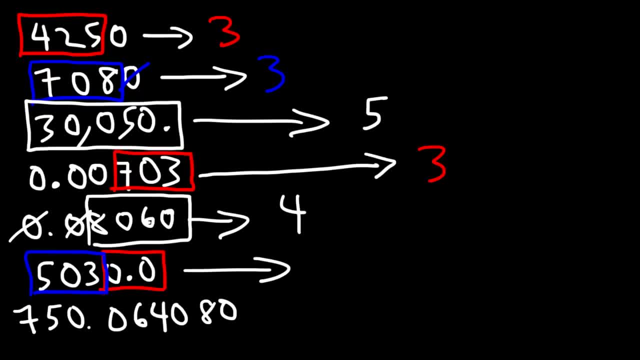 the zero between the three and five. that's always counted. so we have a total of five significant figures. for the last example, all of the zeros in between the nonzero numbers are counted, and since we have a decimal point, the zero to the right is also counted. so everything is counted in this example. so there's let's. 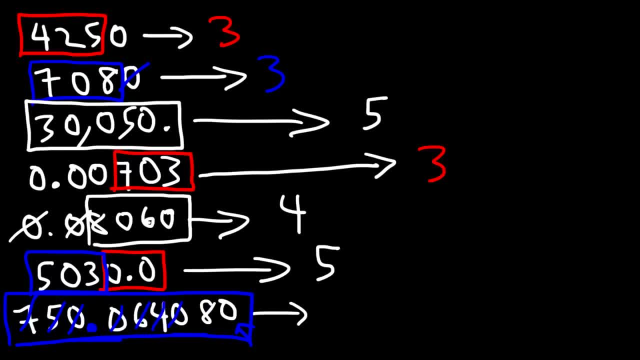 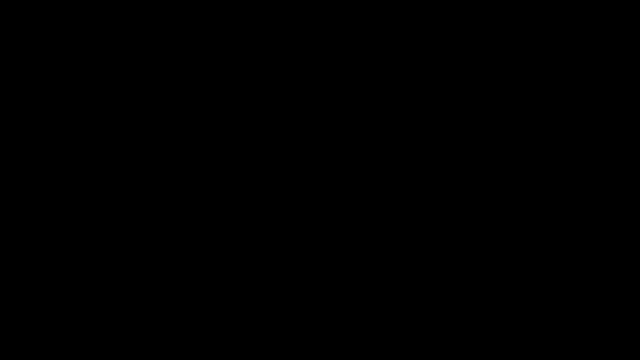 see one, two, three, four, five, six, seven, eight, nine. so we have nine significant figures for that problem. now the next thing that you need to be able to do is you need to be able to round a number when multiplying or dividing. so, for instance, let's say, if we're multiplying 4.6 by 3.5 to how can we round our answer with? 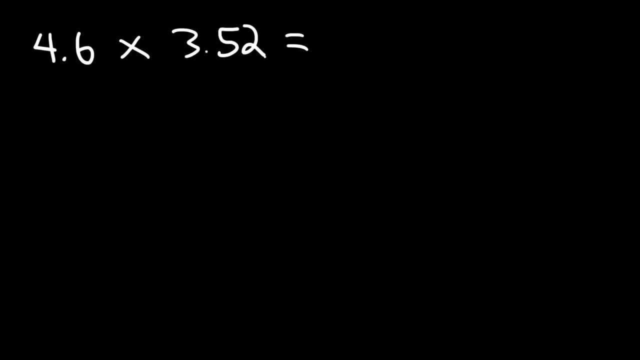 the appropriate number of significant figures. well, the first thing we need to do is perform the calculation. so, 4.6 times 3.5 to. if you type that into your scientific device, your calculator will give you 16.19 to. now how should we round this answer to the? 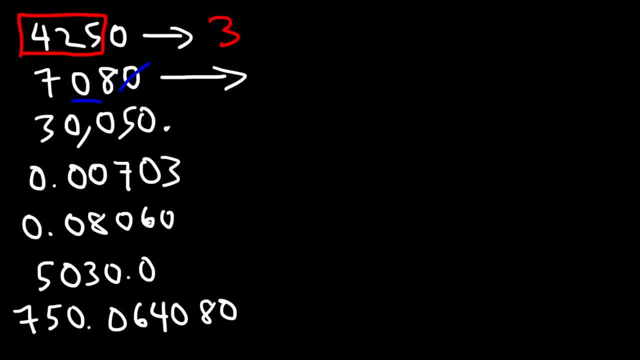 about the zeros in between non-zero numbers. so those zeros we can count. so therefore this answer- I mean this problem- also have a three significant figures. now for the next one. there is a decimal point, so the trailing zero is counted and all of the zeros in between the three and 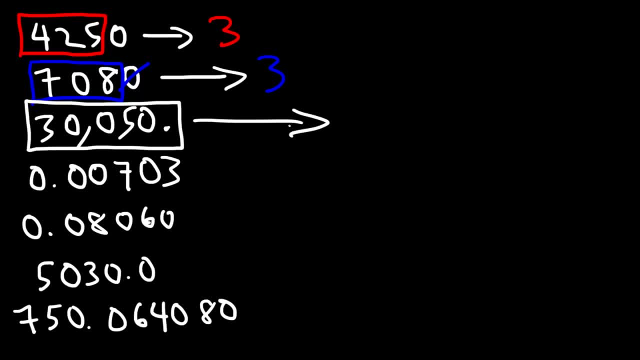 five are also counted. so this example is going to have five significant figures. for the next one, we do have a decimal point, but there are no trailing zeros. we do have some leading zeros, but those will not be counted, so only these three digits will be counted. so there's three significant figures in that number. 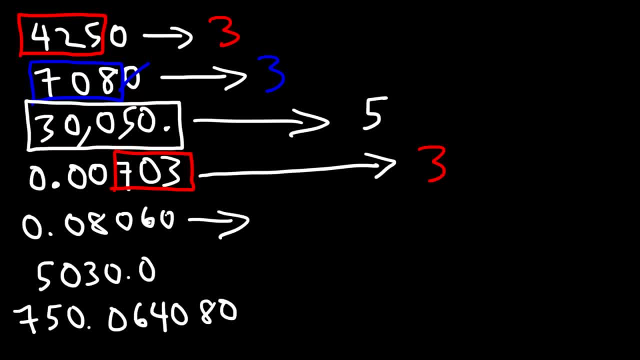 for the next one, we do have a trailing zero which will be counted. the leading zeros will not be counted, so there's only four significant figures now. in the next number, 5030, we have a decimal point, so all of the trailing zeros will be counted, and 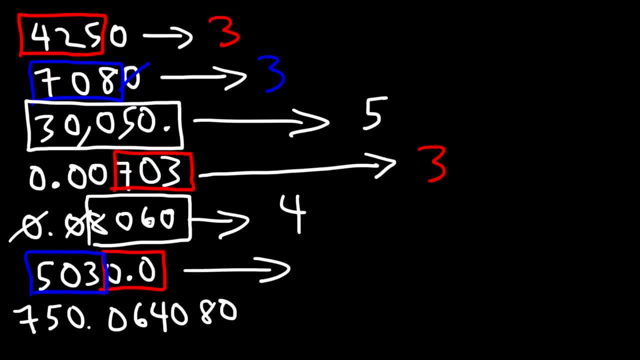 the zero between the three and five. that's always counted. so we have a total of five significant figures. for the last example, all of the zeros in between the non-zero numbers are counted and since we have a decimal point, the zero to the right is also counted. so everything is counted in this example. so there's let's. 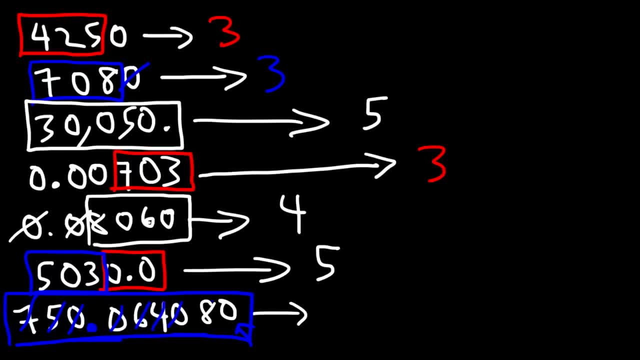 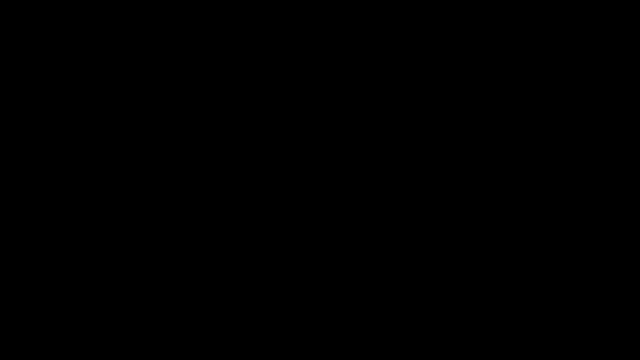 see one, two, three, four, five, six, seven, eight, nine. so we have nine significant figures for that problem. now the next thing that you need to be able to do is you need to be able to round a number when multiplying or dividing. so, for instance, let's say, if we're multiplying 4.6 by 3.5 to how can we round our answer with? 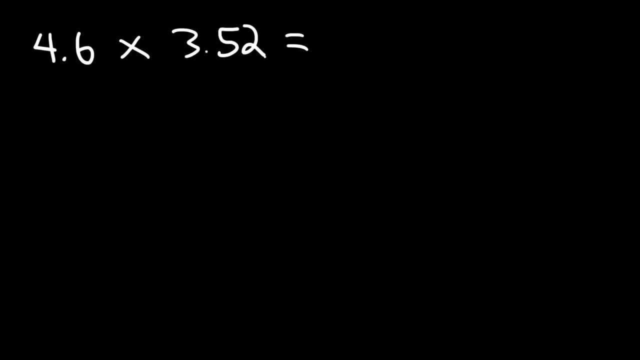 the appropriate number of significant figures. well, the first thing we need to do is perform the calculation. so, 4.6 times 3.5 to. if you type that into your scientific device, your calculator will give you 16.19 to. now how should we round this answer to the? 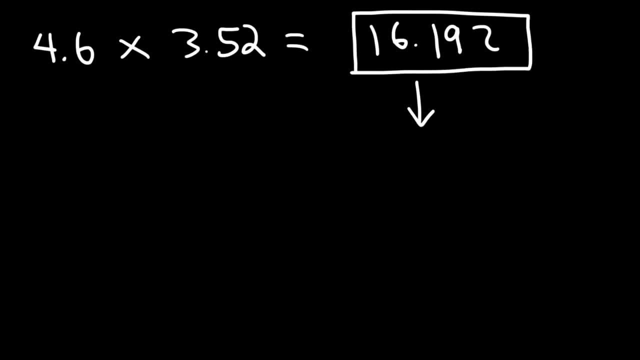 appropriate number of significant figures. what would you say? what we need to do first is we need to determine the least number of significant figures in the first two numbers that we've multiplied already. so in the first number, 4.6, there's two significant figures. in the 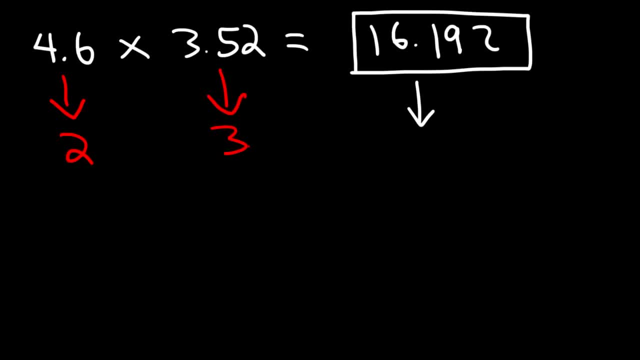 second number, 3.52. there's three significant figures. so when you're multiplying or dividing you need to round your final answer to the least number of significant figures in the original numbers that you use to multiply to get your final answer. so basically, we need to round this answer. 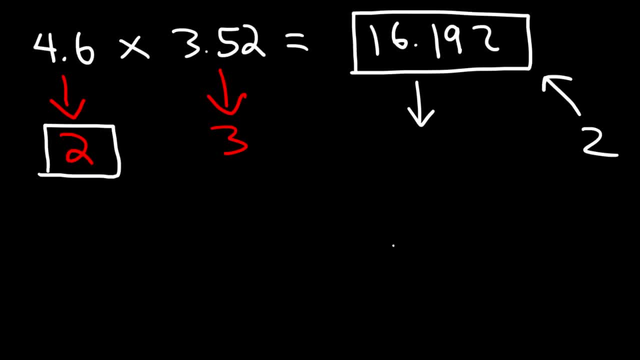 to two sig figs. so, writing it from left to right, we have the first digit, which is a one, and then the second one is a six. now, already this is two significant figures. so the last number that we need to look at is the six. should we keep it at six or should we? 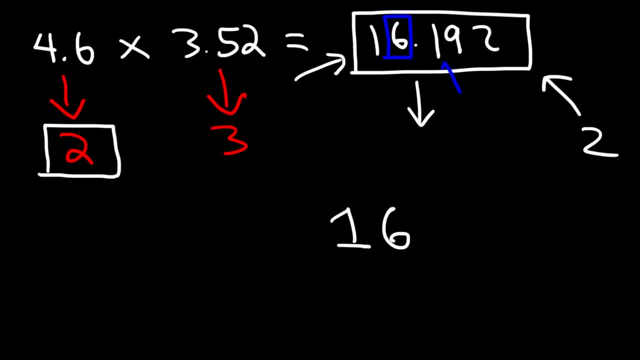 round it up to seven, and so we need to look at the next number. if it's five or more, then we need to round the six to a seven. if it's four or less, then we're going to round down, we're going to keep the six, and because it's four or less, 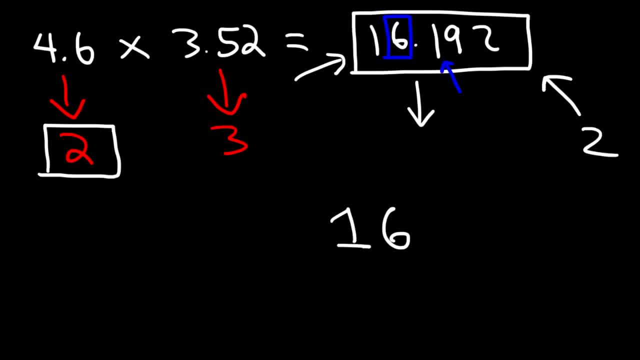 it's one we're going to round down. so our answer is 16 rounded to the appropriate number of sig figs. now let's work on some other examples. let's multiply five point six, four by three point, or rather, let's choose a higher number by twelve point four, five, eight. and let's divide ninety six point seven. 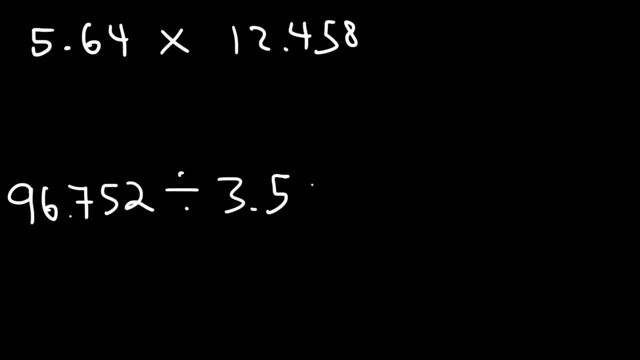 five, two by three point five, four, one. go ahead and try those two examples around your answer to the appropriate number of significant figures. so first let's type this in the calculator: so five point six, four times twelve point four, five, eight. so the calculator gives us seventy point two, six, three, one, two. 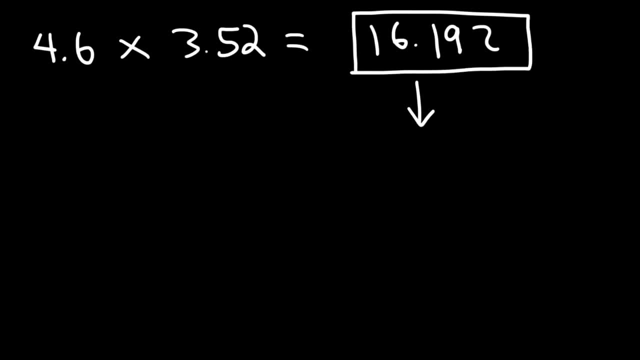 appropriate number of significant figures. what would you say? what we need to do first is we need to determine the least number of significant figures in the first two numbers that we've multiplied already. so in the first number, 4.6, there's two significant figures. in the 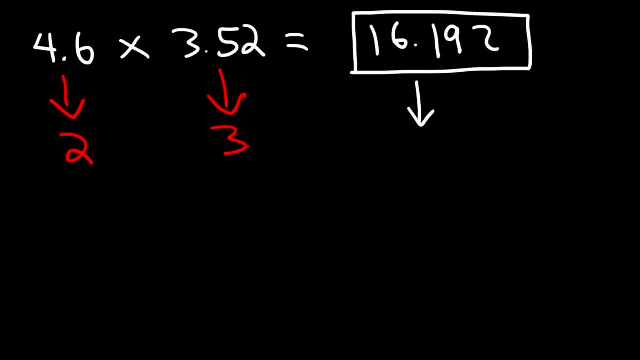 second number, 3.5 to, there's three significant figures. so when you're multiplying or dividing you need to round your final answer to the least number of significant figures in the original numbers that you use to multiply to get your final answer. so basically, we need to round this answer. 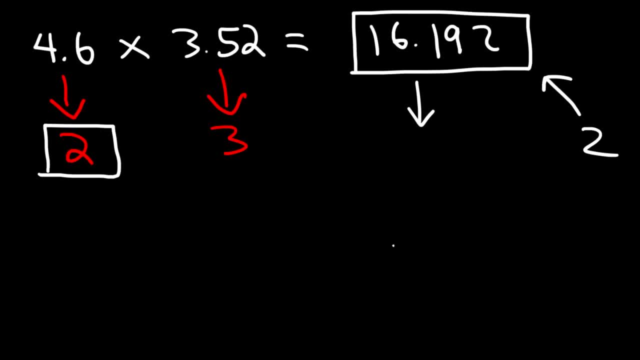 to two sig figs. so the last number that we need to look at is the six. should we keep it at six or should we brought it up to seven? and so we need to look at the next number. if it's five or more, then we need to round the six to a seven. if it's four or less, 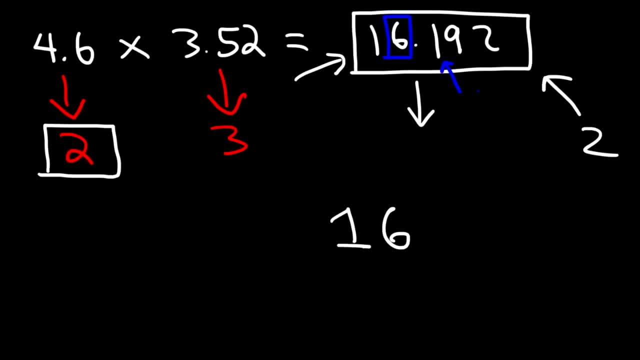 then we're going to round down. we're going to keep the six and because it's four or less, it's one, we're going to round down. so our answer is 16 rounded to the appropriate number of sig figs. now let's work on some other examples. let's 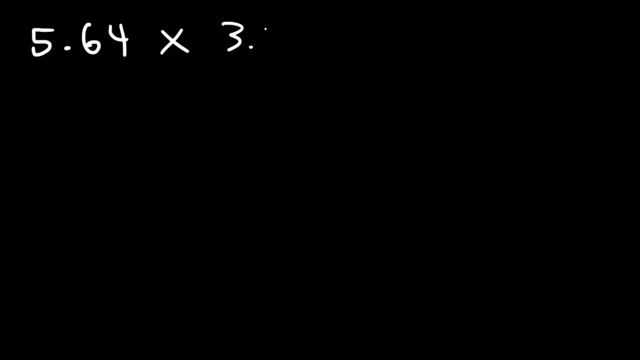 multiply 5.64 by three point, or rather, let's choose a higher number by 12.458 and let's divide ninety six point seven, five, two by three point five, four, one. go ahead and try those two examples round your answer to the appropriate number of significant. 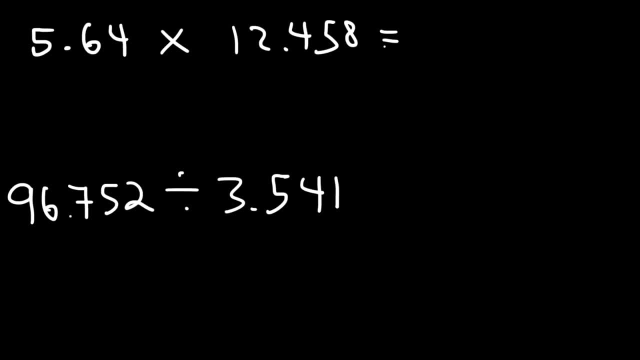 figures. so first let's type this in the calculator. so 5.64 times 12.458, so the calculator gives us seventy point two, six, three, one two. now the first number has three significant figures and the second number has five significant figures. so we have to round our answer. 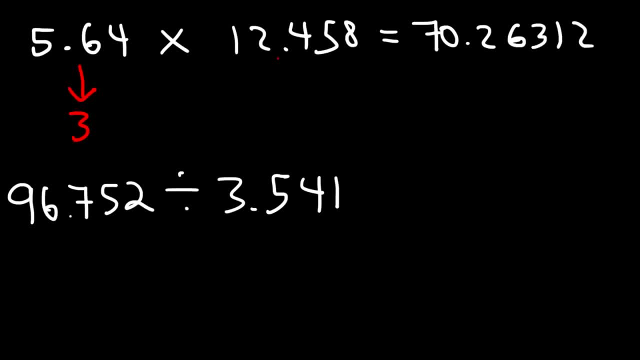 now, the first number has three significant figures and the second number has five significant figures. so we have to round our answer to the least number of significant figures. so that's three. so how can we round seventy point two, six, three, one, two to three significant figures? so we're going to 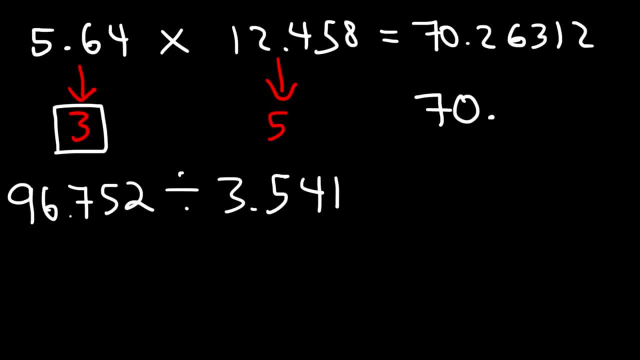 need the first number, the second one and the third one. should we keep it a two or should we round it up to a three? looking at the next number to the right of the two, it definitely falls in the category of five or more. so that tells us that we need to round up. we need to round a two to a three. so the 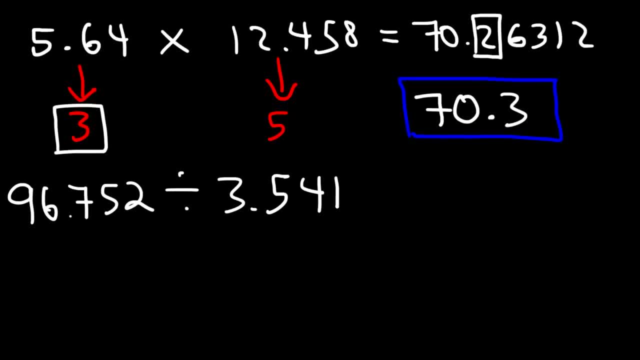 answer for this example is 70.3 and it has three significant figures. this answer has a total of seven significant figures. now let's try the next example. so let's begin by dividing ninety six point seven, five, two by three point five, four, one, and so you. 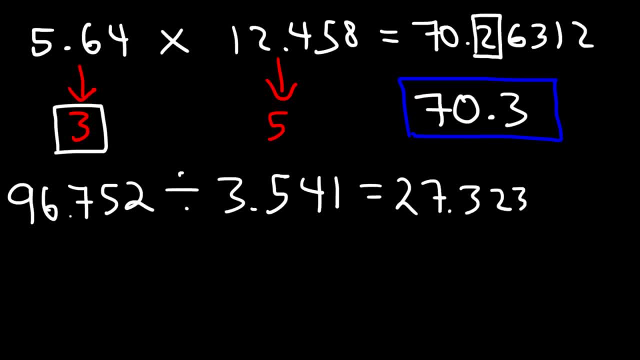 should get twenty seven point three, two, three, three, five, 498. now the first number has five significant figures and the second number has four. so, like always when multiplying or dividing, you need to round your final answer to the least number of significant figures, in this case for. so, looking at the fourth digit or the fourth significant figure, 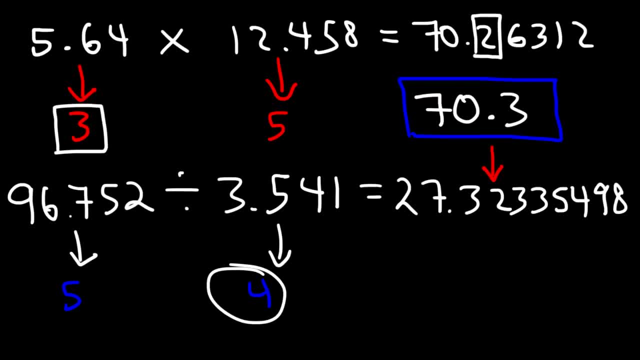 started from the left. should we keep it at a two or should we round it up to a three? so, looking at the next number, it falls in the category of four or less, so we're going to keep the two. so our final answer is 27.32. now let's talk. 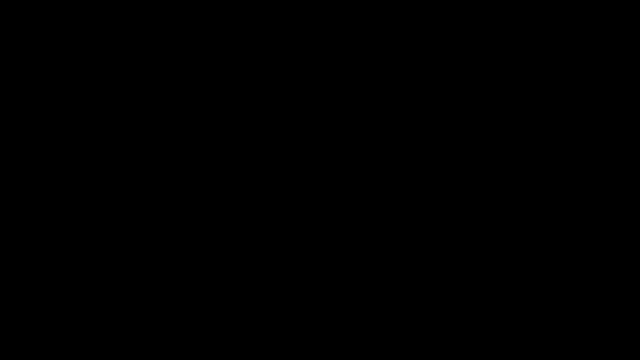 about addition and subtraction, but mostly addition. so let's say, if we wish to add two point three, six plus twelve point one, how can we round our answer to the appropriate number of significant figures? so if we add these two numbers, this will give us fourteen point four, six. but what should we do here for this? 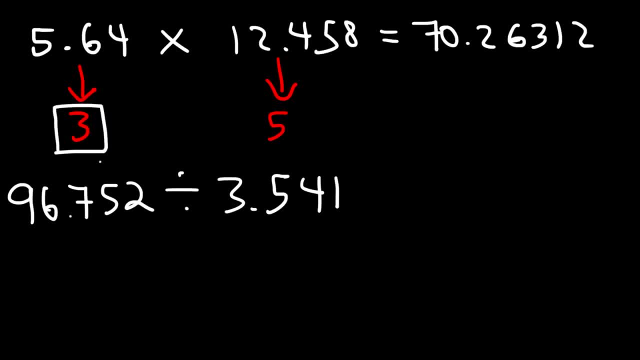 to the least number of significant figures. so that's three. so how can we round seventy point two, six, three, one, two, two, three significant figures. so we're going to need the first number, the second one and the third one. should we keep it a two or should we round it up? 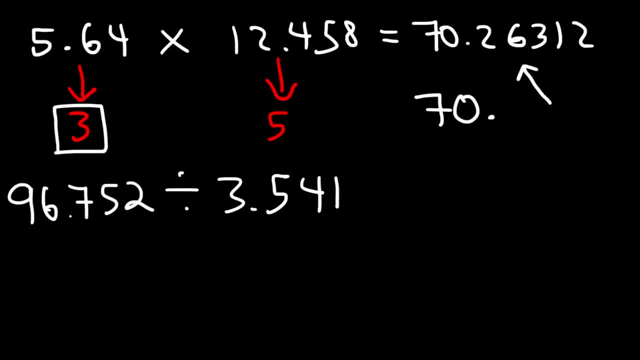 to three. looking at the next number to the right of the two, it definitely falls in the category of five or more. so that tells us that we need to round up. we need to round it to two or three. so the answer for this example is 70.3 and it. 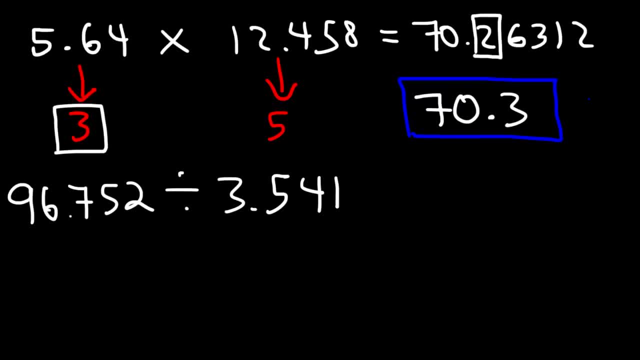 has three significant figures, this answer has a total of seven significant figures. now let's try the next example. so let's begin by dividing ninety six point seven, five, two by three point five, four, one, and so you should get twenty seven point three, two, three, three, five, four, nine, eight. 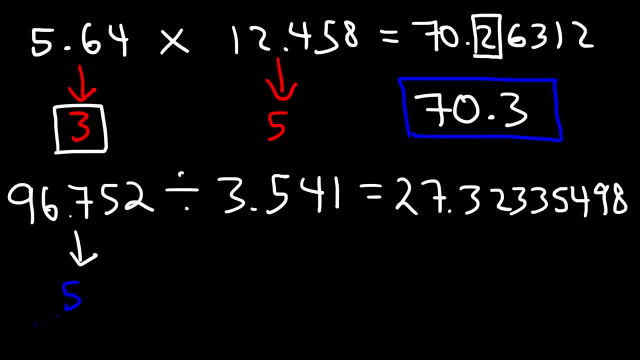 now, the first number has five significant figures and the second number has four. so, like always when multiplying or dividing, you need to round your final answer to the least number of significant figures, in this case four. so, looking at the fourth digit or the fourth significant figure starting from the left, should we keep it at a two or should we round it up to a? 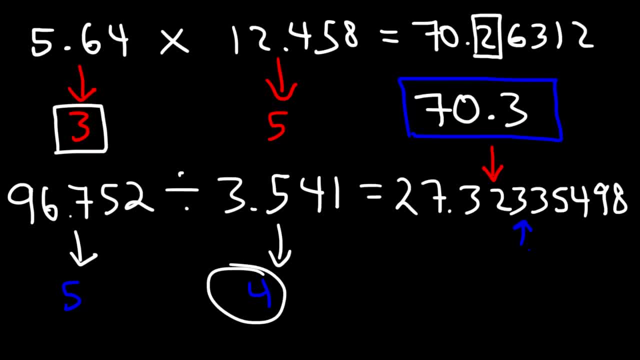 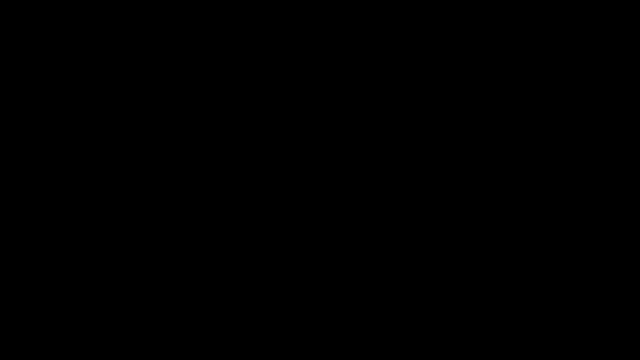 three. So, looking at the next number, it falls in the category of 4 or less, So we're going to keep the 2.. So our final answer is 27.32.. Now let's talk about addition and subtraction, but mostly addition. 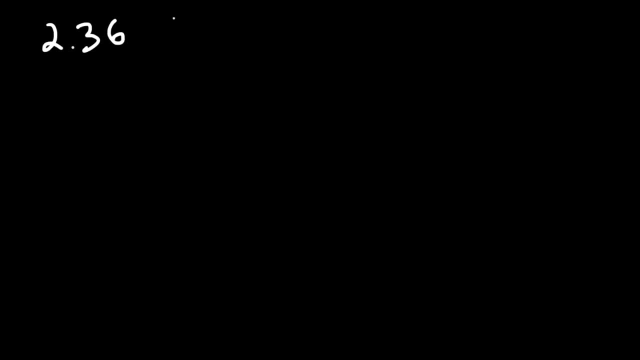 So let's say, if we wish to add 2.36 plus 12.1.. How can we round our answer to the appropriate number of significant figures? So if we add these two numbers, this will give us 14.46.. But what should we do here? 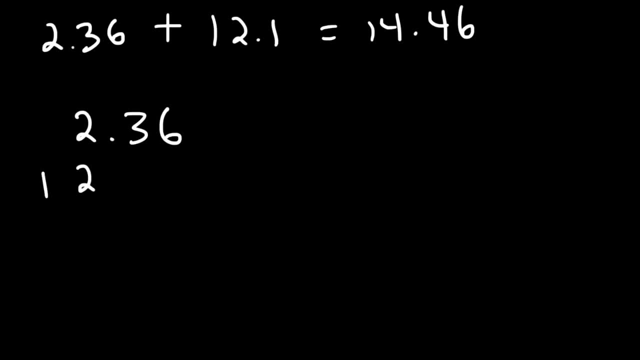 For this type of problem, it's better to write the problem like this: Now you need to round your final answer to the least number of digits to the right of the decimal point. So what I like to do is draw a line, Because for 12.1, there is no number to the right of the 1.. 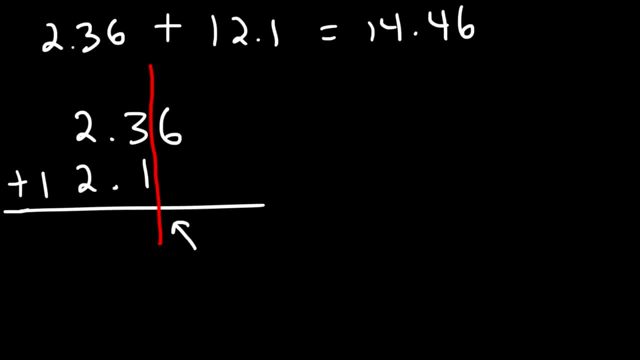 And so we're not going to have any number to the right of this line. But now, if we add the two numbers, it's going to give us 14.46.. So what we're going to do is we're going to keep this significant figure. 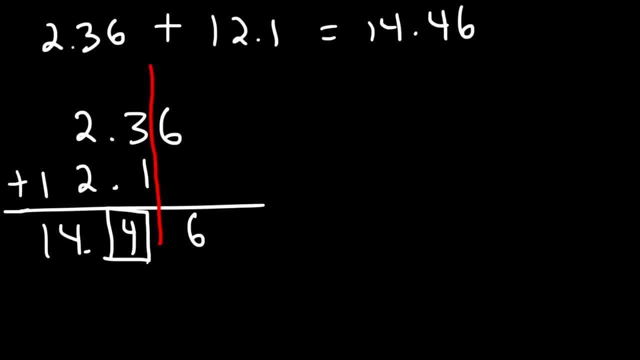 but we need to determine if it should stay a 4 or if we should round it up to a 5.. Looking at this number, it's greater than 5, so we need to round this number up, So our answer is going to be 14.5.. 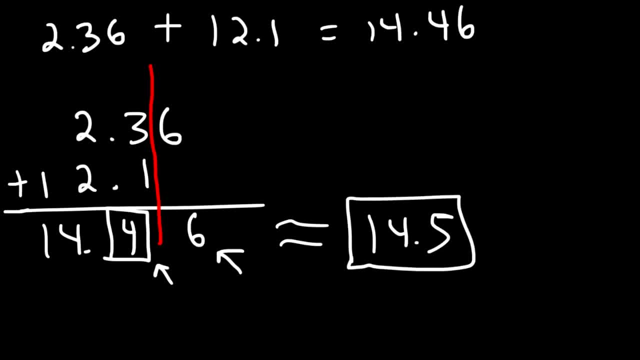 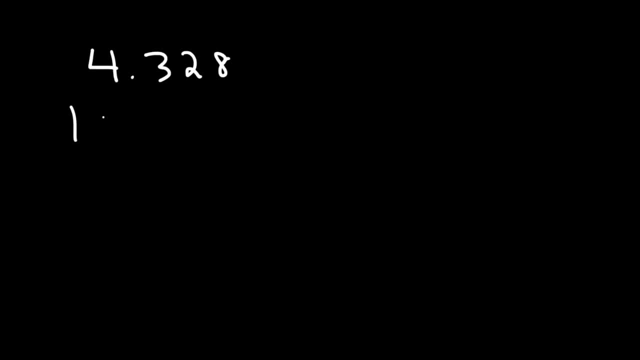 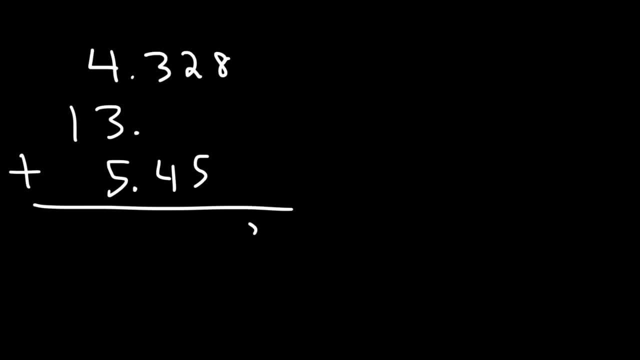 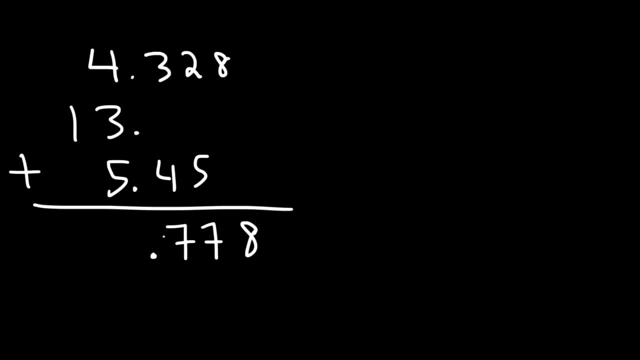 3 plus 4 is 7.. And then 4 plus 3 plus 5 is 12.. Carry over the 1., And 1 plus 1 is 2.. So we get 22.778.. Now what should we do next? 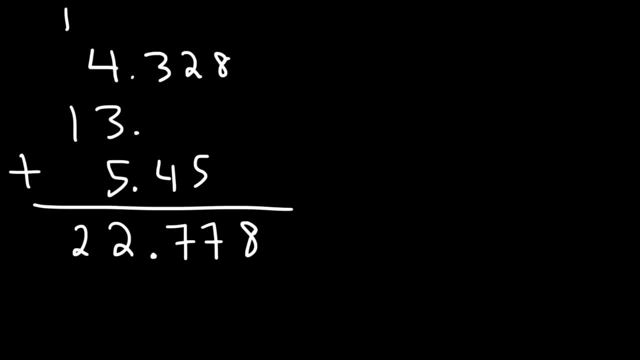 How can we round it? So what we need to do now is determine which number has the least number of digits to the right of the decimal point, And so that's the second number. So we're going to draw the line here, because it has nothing on the right side of that line. 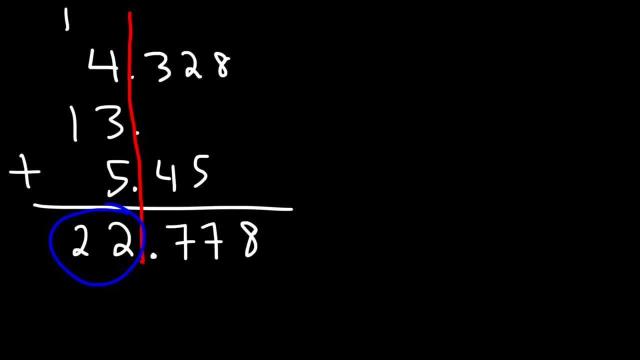 So, therefore, our final answer should only contain these two digits, But we're going to use the 7 to determine what we need to do to the 2.. Should we keep it a 2 or round it up to a 3? Well, 7 is more than 5.. 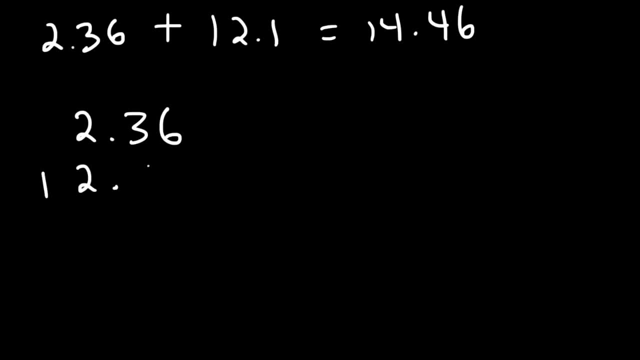 type of problem. it's better to write the problem like this: now you need to round your final answer to the least number of digits to the right of the decimal point. so what I like to do is draw a line, because for twelve point one, there is no number to. 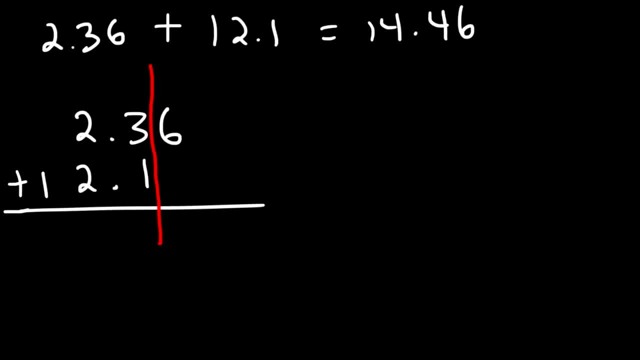 the right of the one, and so we're not going to have any number to the right of this line. but if we added two numbers, it's going to give us 14.46. so what we're going to do is we're going to keep this significant figure, but we need to. 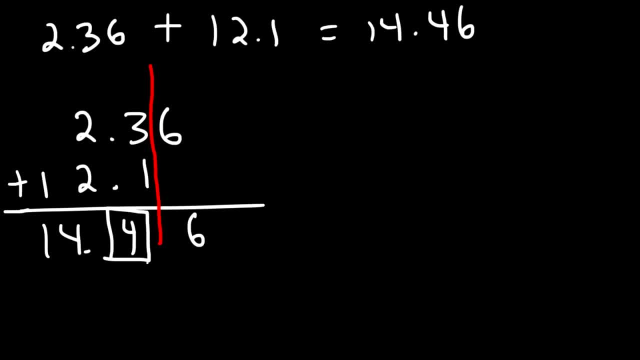 determine if it should stay a four or if we should round it up to a five. looking at this number, it's greater than five, so we need to round this number up. so our answer is going to be 14.5, and that's how you supposed to do it. when adding or. 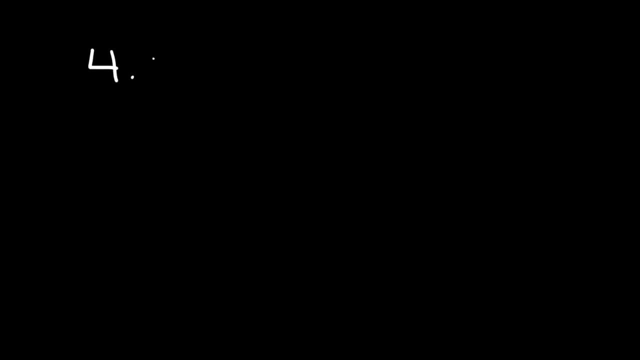 subtracting. let's try another example: 4.3 to 8 plus 13 plus 5.45. so go ahead and try that problem. well, first we need to add, so we have an 8, 2 plus 5 is 7, 3 plus 4 is 7, and then 4 plus 3 plus 5 is 12. carry over the 1 and 1. 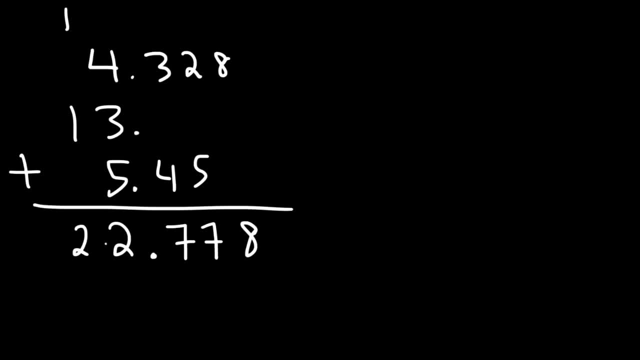 plus 1 is 2, so we get 22.778. now what should we do next? how can we round it? so what we need to do now is determine which number has the least number of digits to the right of the decimal point, and so that's the second number. so we're going. 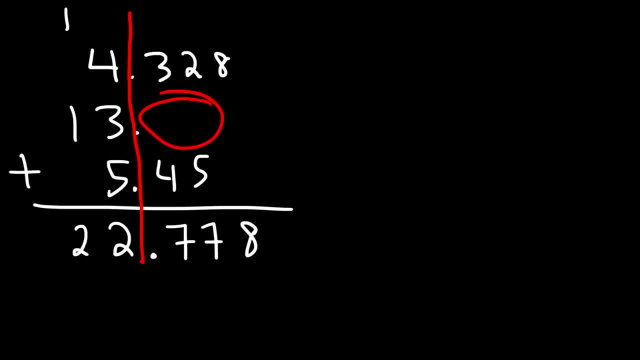 to draw the line here, because it has nothing on the right side of that line. so, therefore, our final answer should only contain these two digits, but we're going to use the 7 to determine what we need to do to the two. should we keep it a two or rounded up to a three?